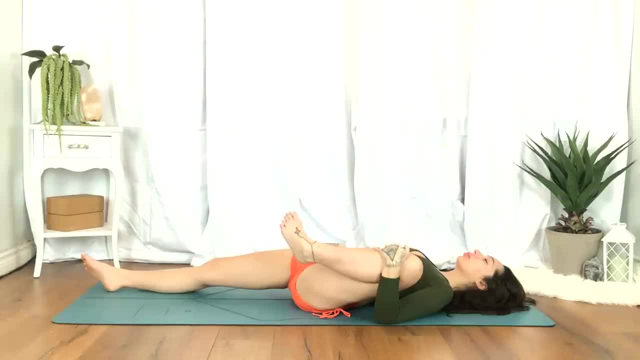 And again, you can rest right here if you'd like to get a little bit of opening in the hips. here You can start to draw that left knee towards the left armpit And we'll release, straightening the legs, reaching the arms up overhead, so really getting. 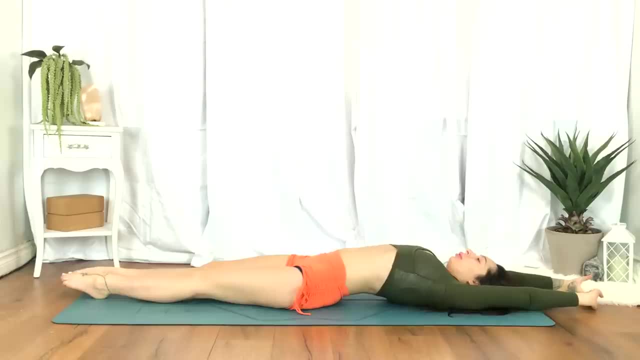 a good stretch here. Feel free to yawn- I know it has that effect And we'll go ahead. whenever you're ready to bend the knees, plant the feet on the mat, hands by your sides, palms facing down On an inhale, we'll begin to lift the hips for bridge pose. 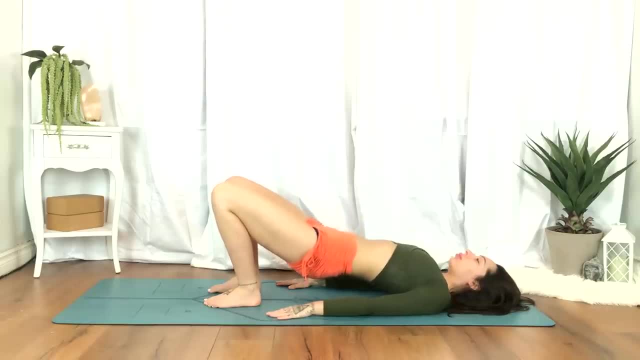 And, on an exhale, releasing the hips back down. We're going to do this a few more times. Continue sinking breath with movement, going at your own pace here, Just lifting the hips as high as you comfortably can. We're not trying to get a deep, deep backbend here, just to get into the core, into the. 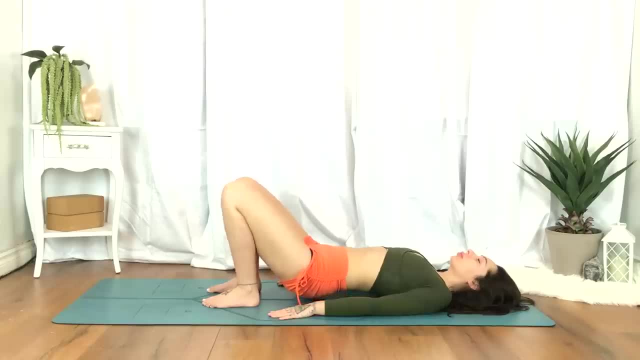 back muscles a little into the spine. Good, Good, Perfect. Releasing the hips back down towards the mat, Begin hugging the knees towards the chest, Grabbing the outer edges of the feet, Maybe rocking side to side, Massaging the back muscles a little. 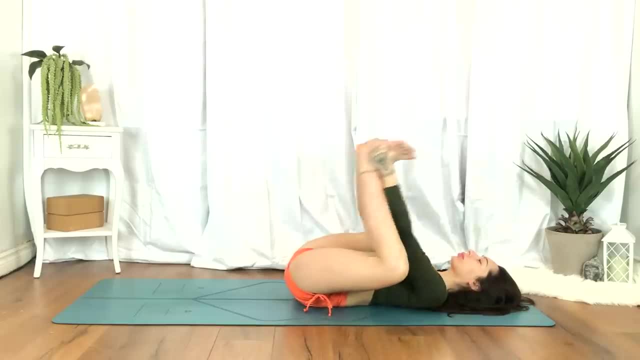 Or, if you'd like, you can come right into your happy baby pose by opening the feet Again option to rock side to side, feeling that connection of your back pressing into the mat, And we'll release. Come to seated. 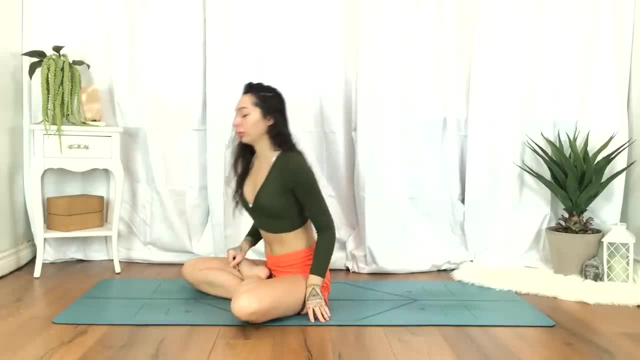 Begin to find some movement in the neck, maybe circulating or rocking the head side to side, maybe ear to shoulder, ear to shoulder, Just a gentle movement. here We'll come back to center, Begin circulating the shoulders Again, finding some stillness. 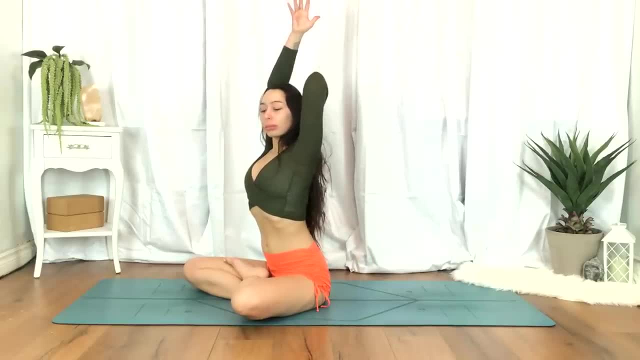 We'll inhale the hands up overhead, Exhale. drop the left hand behind your head, Right hand resting on that left elbow. Now this could be a little intense, so, if so, just grab opposite wrists. We'll sit tall here. 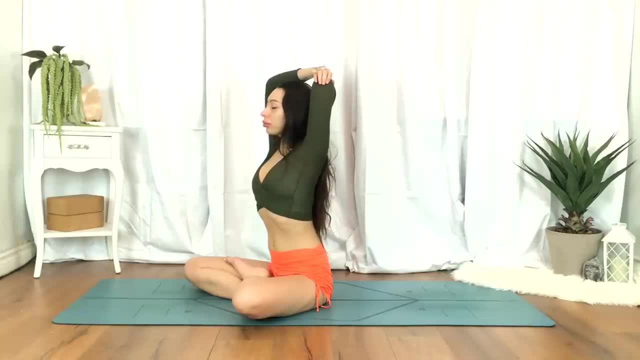 avoiding any hunching in the upper, back or neck, Switching sides: left hand to the right elbow, right hand just falls just behind the head. Sit tall, Take a deep breath in two, three, four, five, six, seven, eight, nine, 10.. 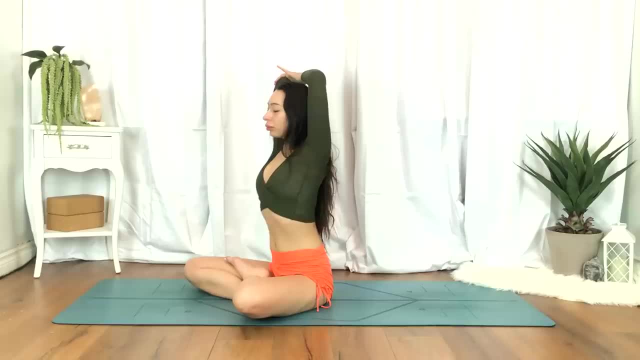 Good Exhale release, Shake it out. take a moment here. When you're ready, hands to heart center. We'll interlace the fingers, Draw a big circle with the palms of your hands and just really getting into the waist, into. 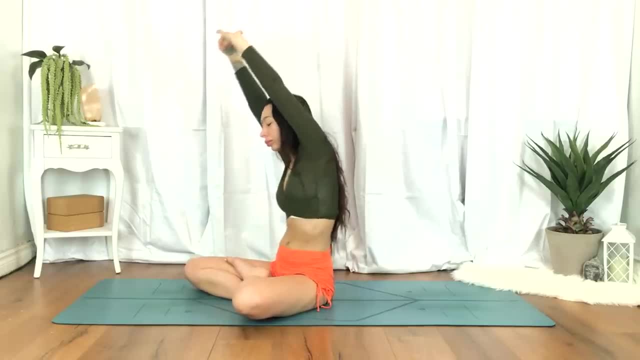 the shoulders here, in the upper back, all the way through the spine. So have fun here, Just feel the movement. Move like nobody's watching, Just you and your mat. Starting back to centre, take the left hand to the mat, right hand reaches up overhead.